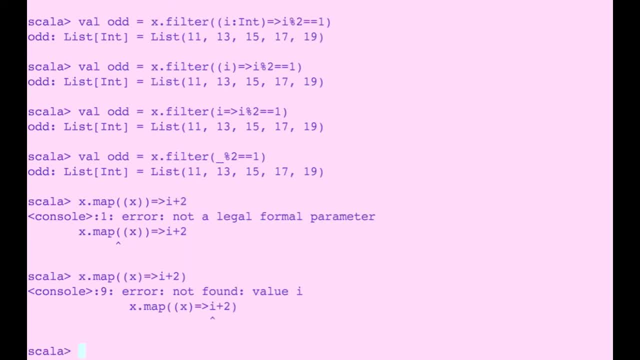 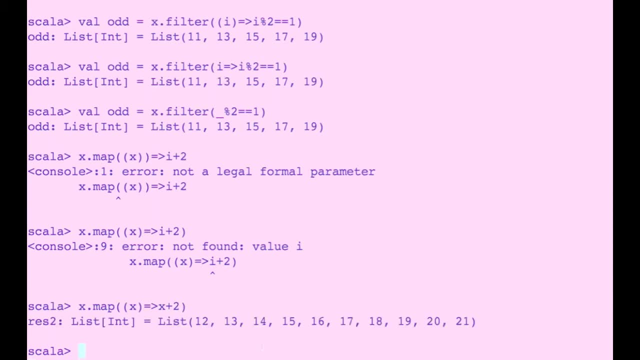 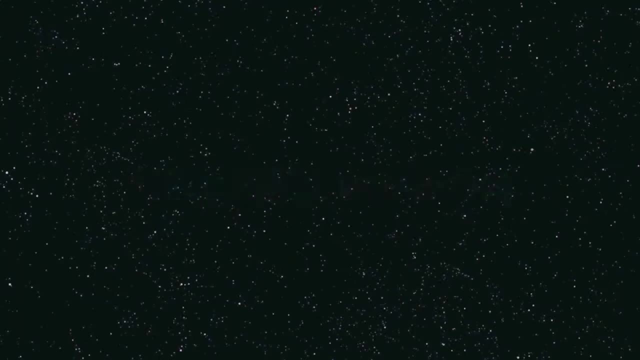 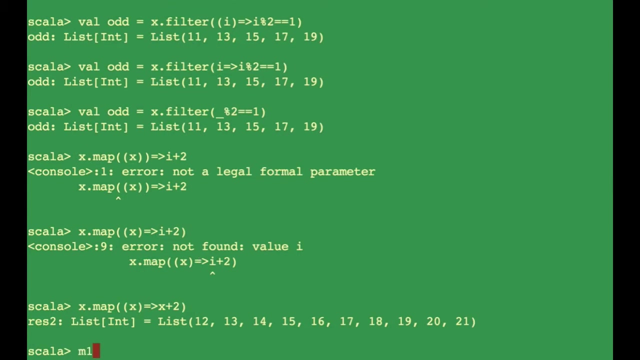 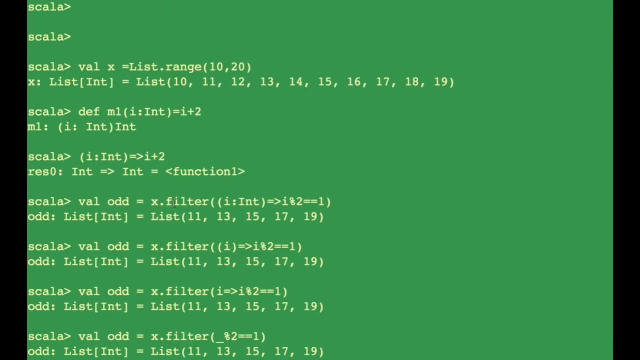 In this list. So 2 is being added. The method: what we have created is M1.. Ok, If we add 2. It will give me 4. Because the definition of method is i plus 2. Let's define this one also. 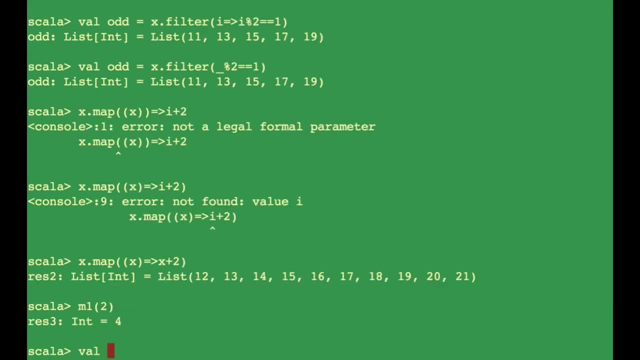 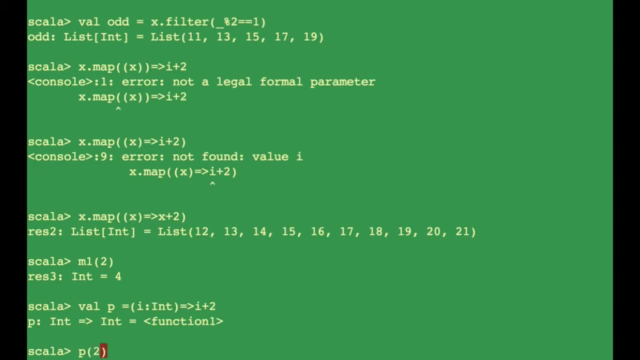 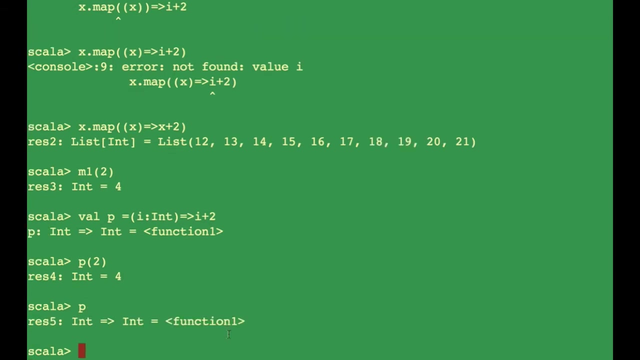 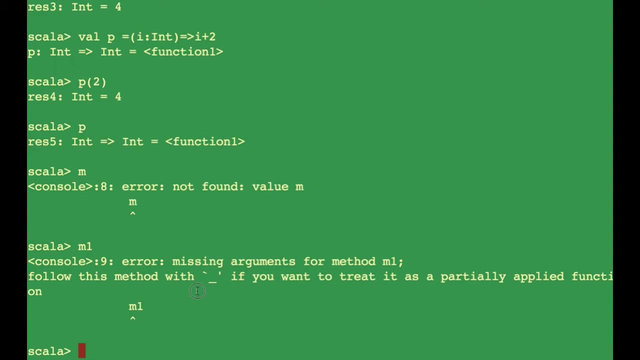 To define this, Let's say p is equal to, So p will take 2.. If we give only p, It will give the function M1.. Ok, Cannot be a final value. So the function, So this function can be a final value. 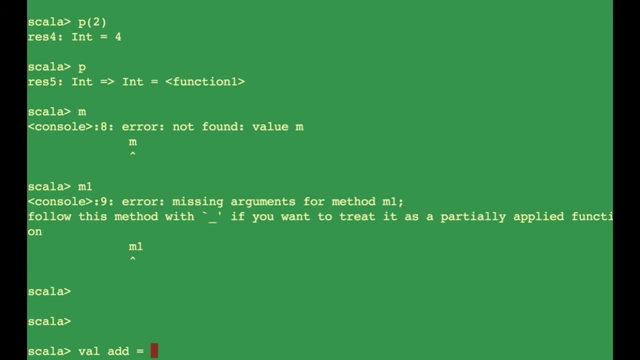 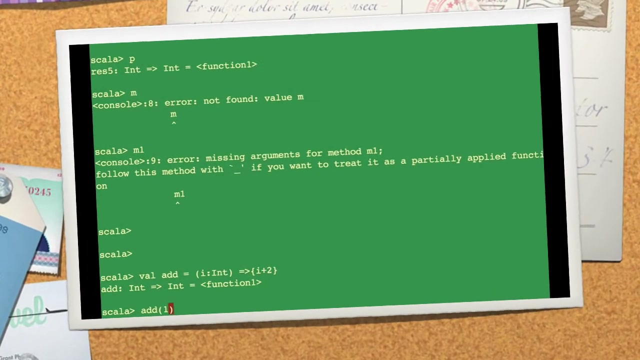 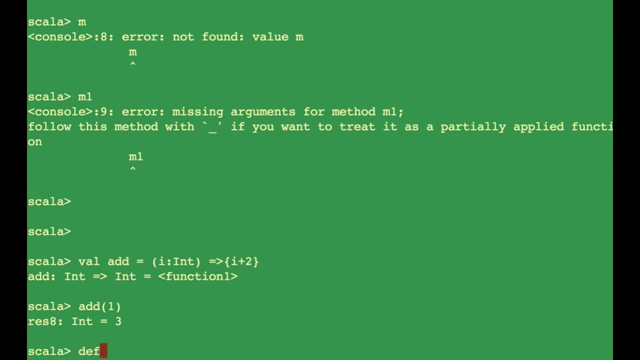 It also has 2. here I will create a new one. Start salty only, And then: □ Now get back to fn1, value 123.. □ fn1.. □ Now it is crack-free. So you have created one function, so now create a method also. 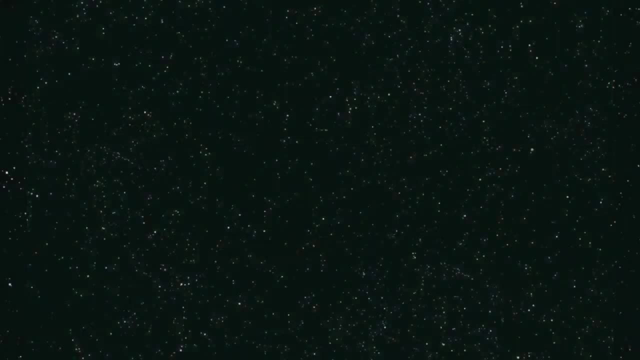 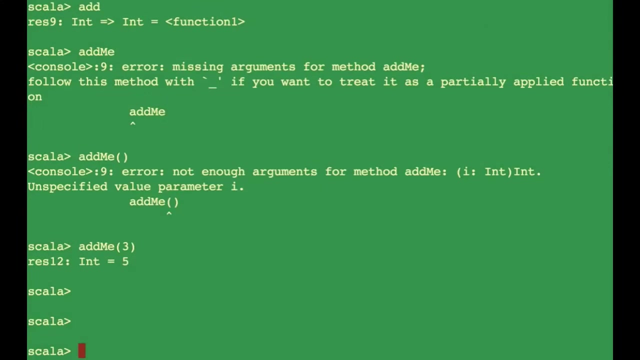 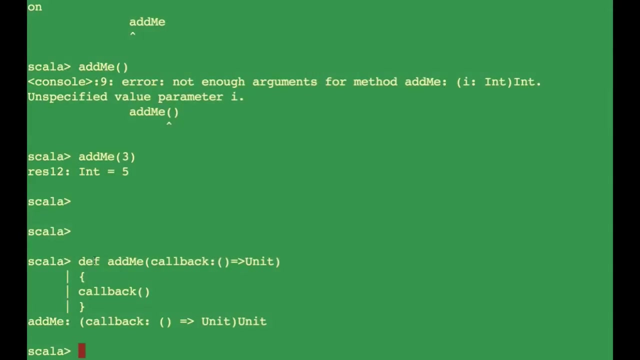 so let's say add, now we will see method that take a single function as method parameter. let's say: I have a add me function- ok, so we have created a method. and let's say: I have a add me function- ok, so we have created a method.